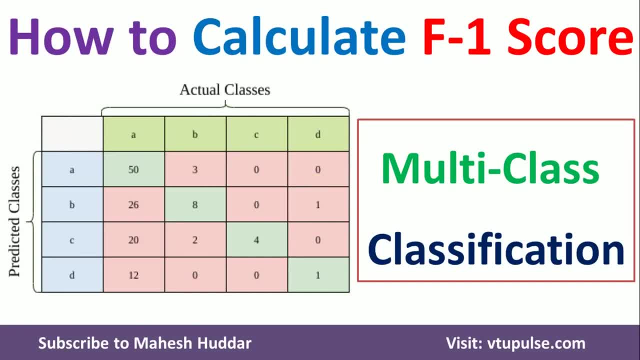 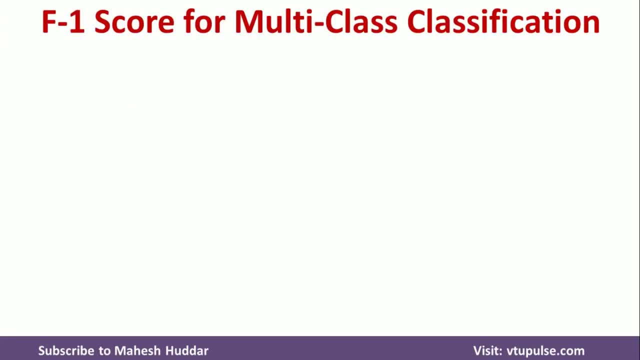 Hi, welcome back. In this video, I will discuss how to calculate F1 score for multi-class classification. When it comes to evaluating the performance of any machine learning model, we use different metrics like accuracy, precision, recall, F1 score and so on. 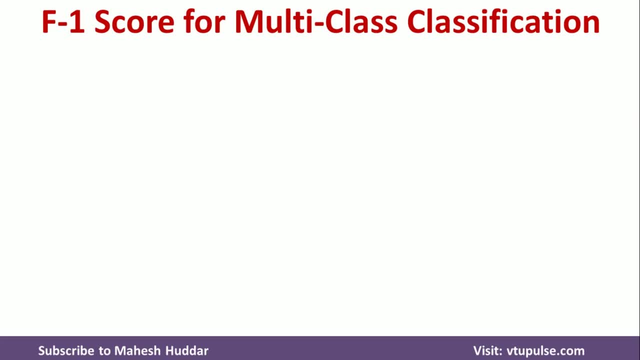 In this video we will understand what is F1 score and how to calculate F1 score for multi-class classification. F1 score is preferable when we have imbalanced class distribution. Let us take an example. We have 1000 examples. Out of 1000 examples, 800 belongs to one class and remaining 200 examples belongs to another class. 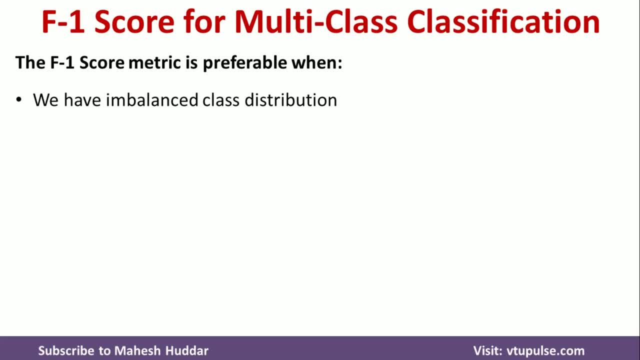 So in this case we have an imbalanced class distribution. In such case we cannot use accuracy performance matrix. In such cases we need to use F1 score So that we will be able to calculate F1 score for multi-class classification. 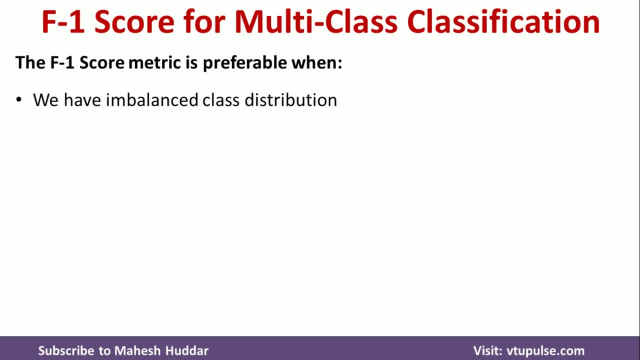 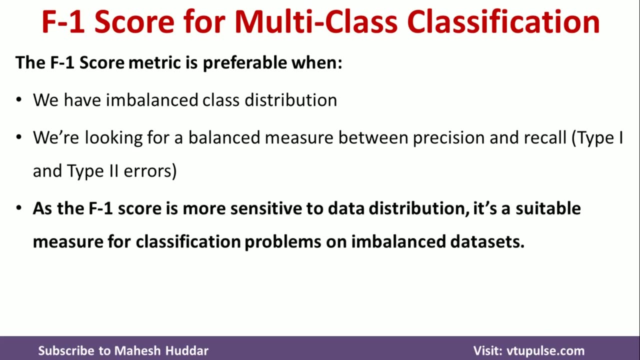 So that we will be able to judge the machine learning model more accurately. F1 score is preferred whenever we want to get the balanced measure between precision and recall. That is nothing but type 1 and type 2 errors. As F1 score is more sensitive to data distribution, it is suitable measure for classification problems on imbalanced datasets. 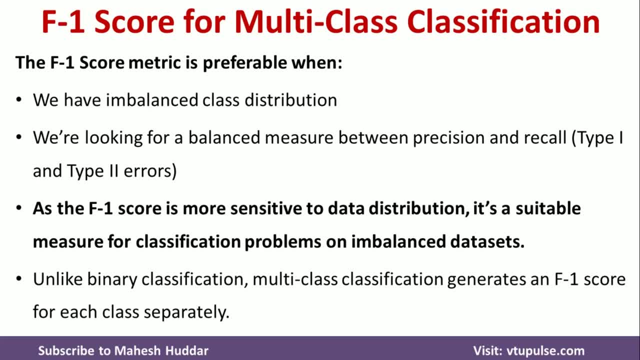 In binary classification we will get overall F1 score for the entire dataset, but when it comes to multi-class classification, F1 score is generated for every class. For example, if we have three classes, F1 score is generated for all the three classes separately, but in binary classification we will get overall F1 score for the entire dataset. 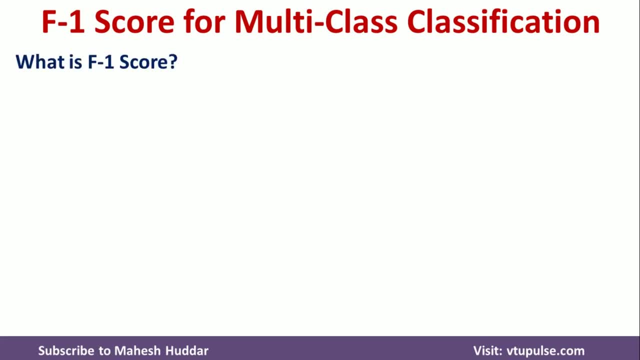 First, we will try to see what is F1 score. Second, we will try to see what is F1 score. Third, we will try to see what is F1 score and what is the formula to calculate F1 score. F1 score is the one of the common measure to rate how successful a classifier is. 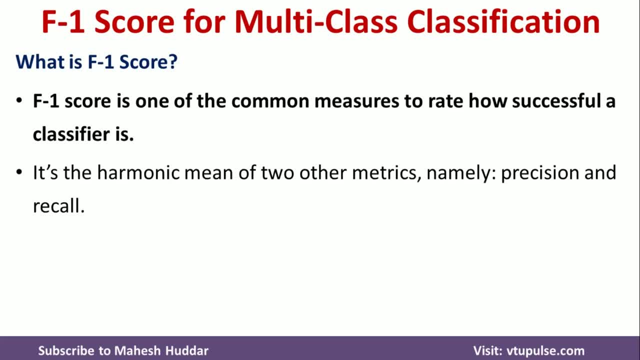 It is the harmonic mean of two other matrix, namely precision and recall. To calculate the F1 score, we can use the formulae that is 2 times precision multiplied by recall. to calculate the F1 score, we can use the formulae that is 2 times precision multiplied by recall. 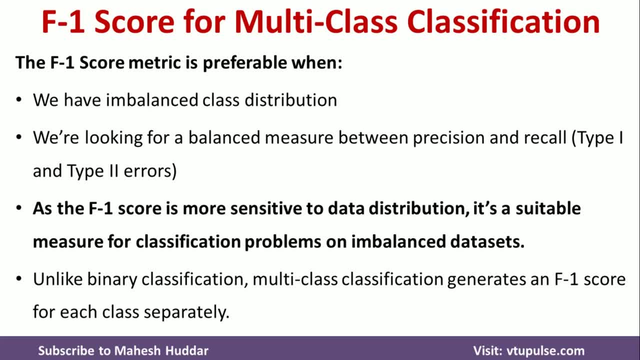 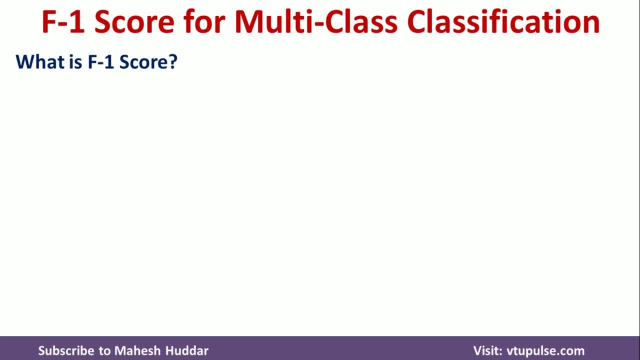 But in binary classification we will get overall F1 score for the entire dataset. First we will try to see what the frame rate is. We will try to see what the frame rate is, what is F1 score and what is the formulae to calculate F1 score. F1 score is one of the 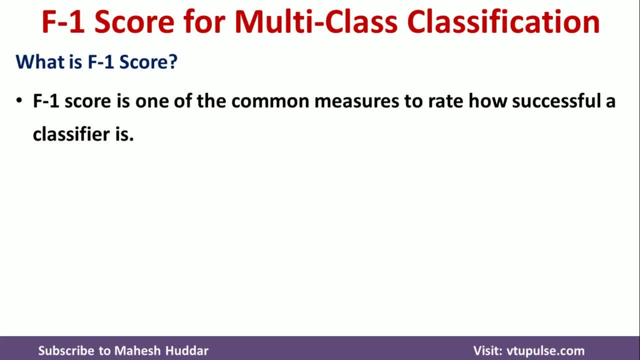 common measure to rate how successful a classifier is. It's a harmonic mean of two other matrix, namely precision and recall. To calculate the F1 score we can use the formulae that is two times precision multiplied by recall, divided by precision plus recall. So, using this particular 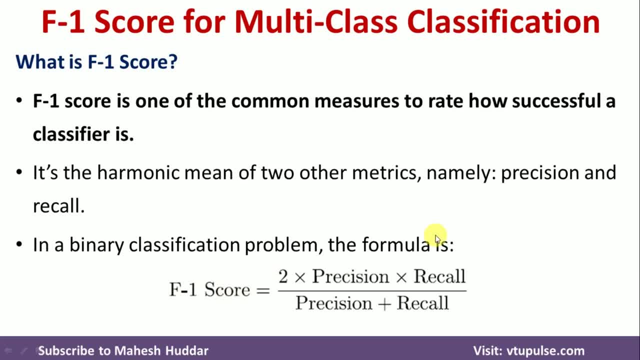 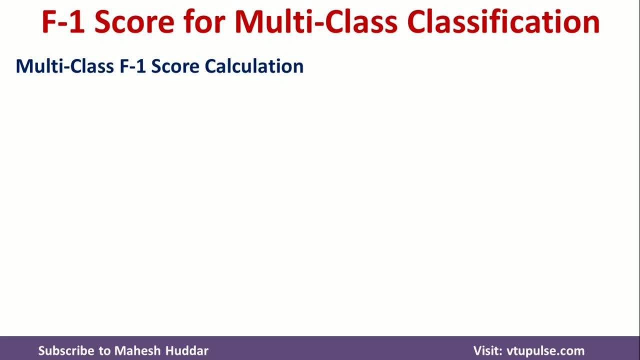 formulae, we can calculate the F1 score for binary classification or, if you are using multi-class classification, we have to calculate this F1 score for every individual class separately. Now we will try to understand how to calculate the F1 score for multi-class classification. 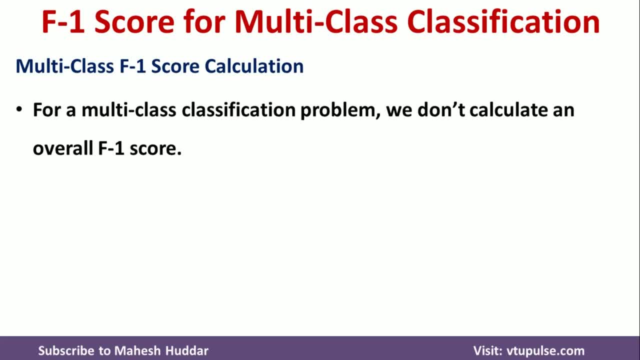 As I said earlier, we have to calculate the F1 score for individual class, like 1 versus rest or something like that. So we need to consider one class at a time and remaining everything will be considered as other side, and then we need to calculate the F1 score. 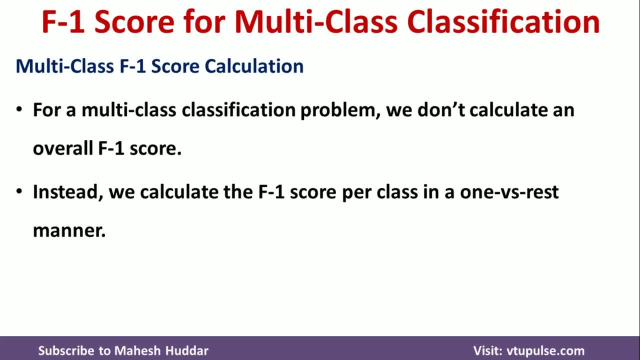 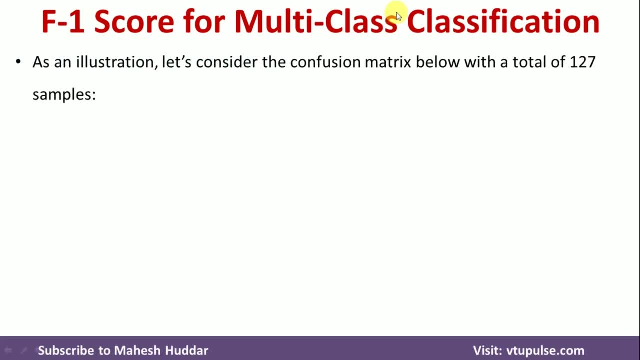 Similarly we have to do it for other classes. in that case, Now we will take a very simple example to understand how to calculate F1 score. We will consider a confusion matrix consisting of 127 samples and four classes, namely A, B, C and D. 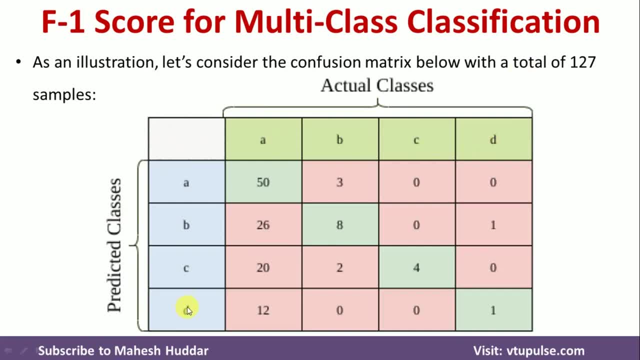 Here we have written the actual classes and here we have written the predicted classes. If you look at this particular 50, the 50 is there are 50 A class. examples are there and they were classified as a here. The meaning is: it's a true A. you can say similarly this: 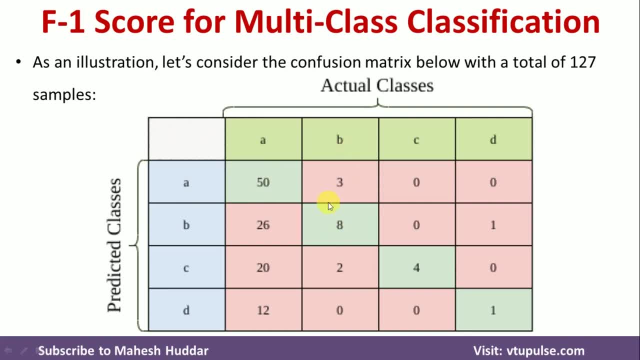 eight represents there are eight B class examples are there, and then we have 8 A class examples. they were classified as B here. Again, these are the true class B examples are correctly classified here, Similarly for C and D. here Now, when it comes to 3, there are 3 B class. 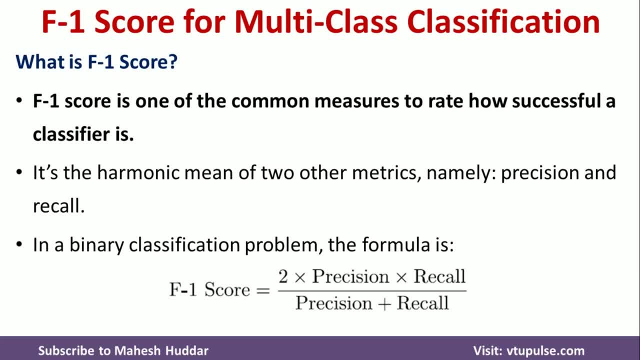 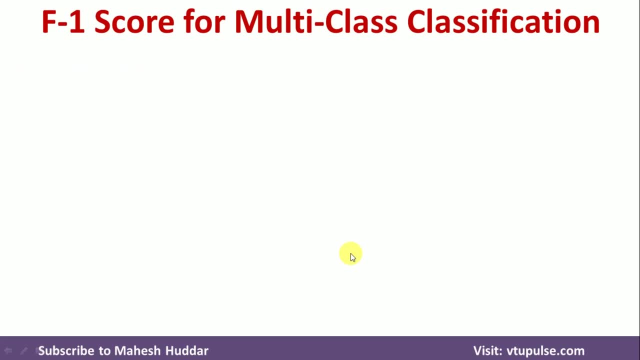 by precision plus recall. so, using this particular formula, we can calculate the F1 score for binary classification. or, if you are using multi-class classification, we have to calculate this F1 score for every individual class separately. now we will try to understand how to calculate the F1 score for multi-class. 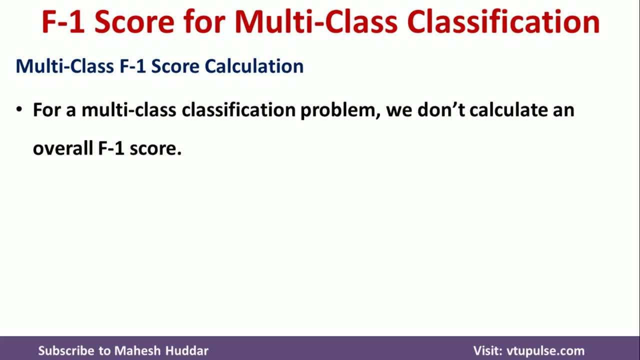 classification. as I said earlier, we have to calculate the F1 score for individual class, like one versus rest or something like that. so we need to consider one class at a time and remaining everything will be considered as other side, and then we need to calculate the F1 score. similarly, we have 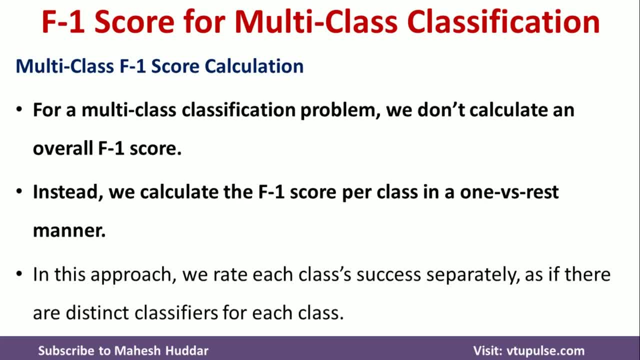 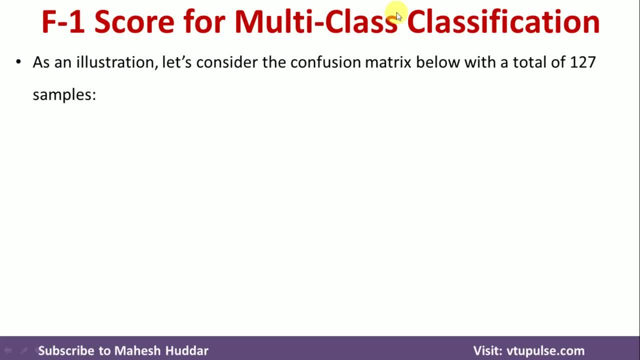 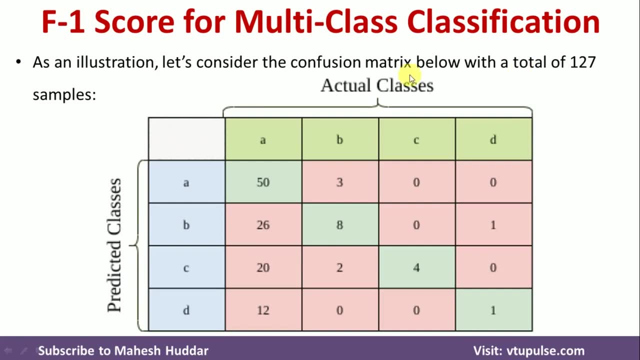 to do it for other classes. in that case, now we will take a very simple example to understand how to calculate F1 score. we will consider a confusion matrix consisting of 127 samples and four classes, namely A, B, C and D. here we have written the actual classes and here we have written the predicted classes. here, if you look at, 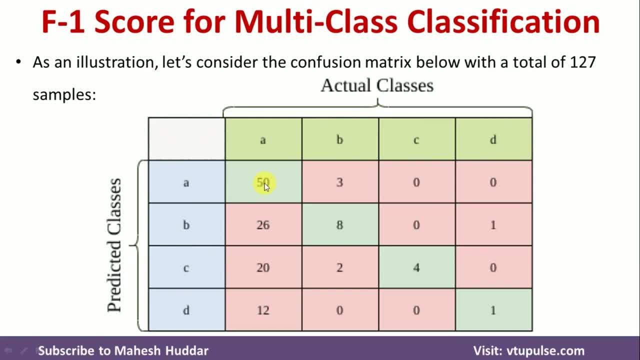 this particular 50. the 50 is there are 50. A class examples are there and they were classified as A here. the meaning is: it's a true A. you can say similarly this: 8, 8 represents there are 8. A class examples are there and they were classified as A here. the meaning is: it's a true A. you can say similarly this: 8, 8 represents there are 8. 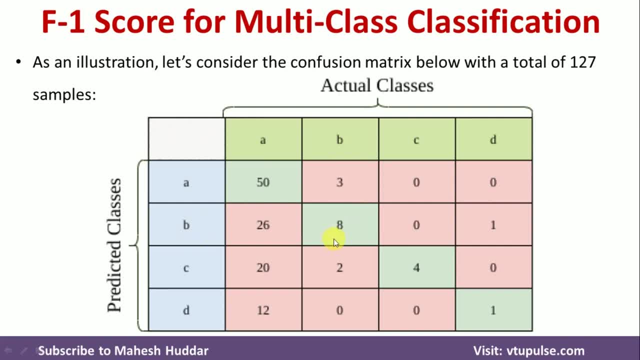 A class examples are there and they were classified as B. here again, these are for 3. there are three B class examples are there, but they were classified as a here. that is nothing but false positive in this case. similarly, if you consider this 26, 26 are of type a and they were classified as B. here it is. 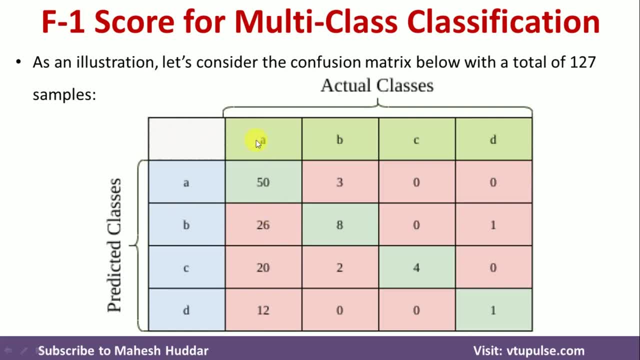 nothing but false negative in this case. actually, they are of type a, but they were classified as b. that's the reason it is called as false negative. these are of type b, but they were classified as a. that is the reason it is called as false positive in this case. similarly for other numbers, you can. 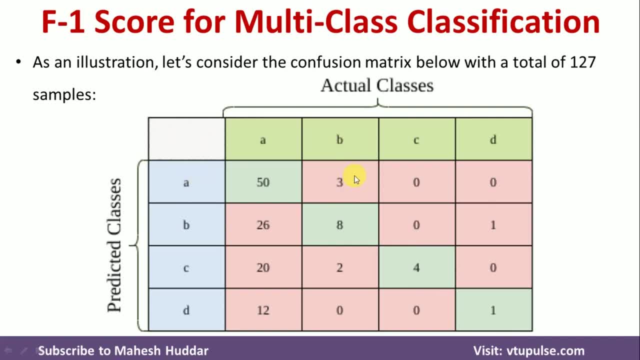 examples are there, but they were classified as A here. That is nothing but false positive in this case. Similarly, if we consider this: 26,. 26 are of type A and they were classified as B here. It is nothing but false negative in this case. Actually, they are of type A, but they were. 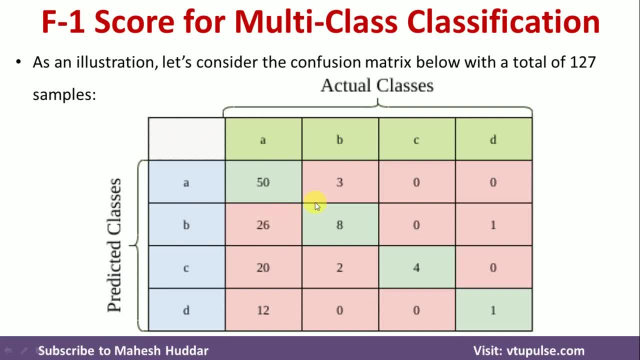 classified as B. That is the reason it is called as false negative. These are of type B, but they were classified as A. That is the reason it is called as false positive in this case. Similarly for other numbers. you can understand which is false positive and which is false negative here. 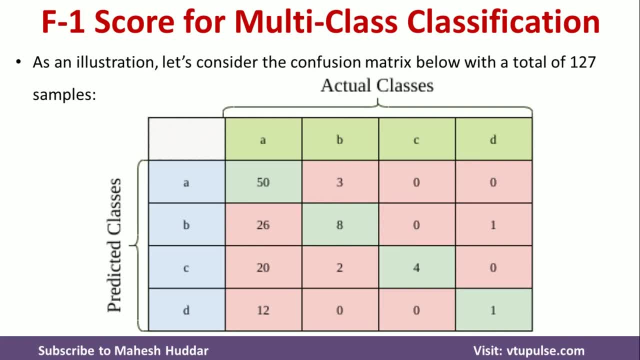 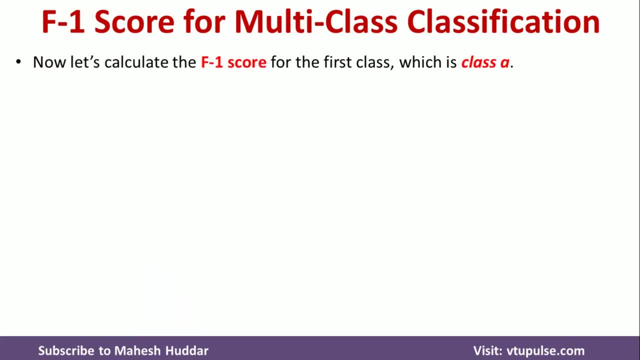 Now what we do is we will consider each class at a time and then we will try to calculate the F1 score here. Now, if I consider the class A first, we need to calculate the precision recall for class A. That is precision. 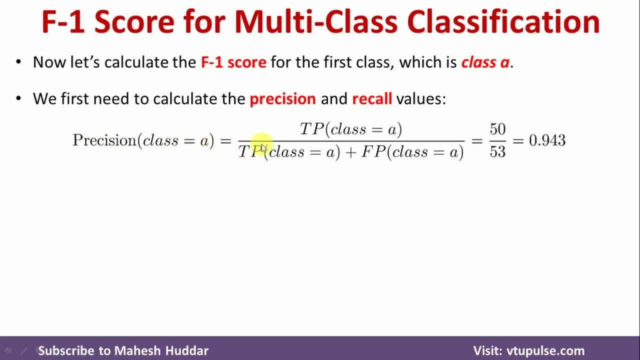 of class A is true positive when class is equivalent to A divided by true positive when class is equivalent to A, plus false positive when class is equivalent to A. So this is a formula to calculate precision: That is true positive divided by true positive plus false positive. 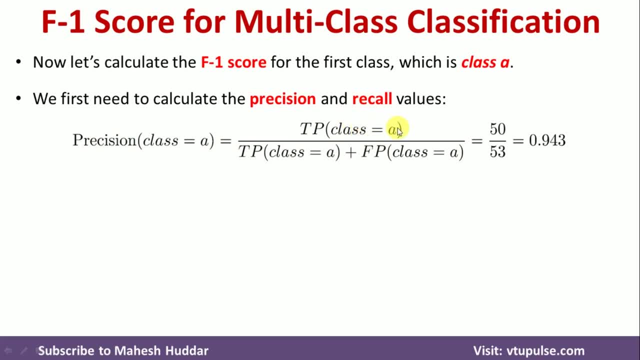 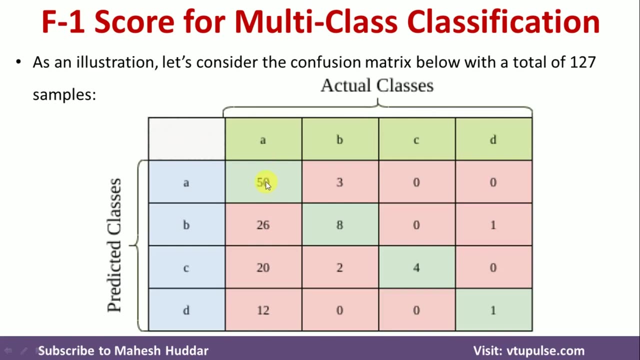 But we have to specify when class is equivalent to A here, Because we have to calculate the F1 score individually. Now what is true positive when class is equivalent to A is: If you look at this particular thing, this one, this 50, is nothing but the true positive when class is equivalent to A. And what we need is: 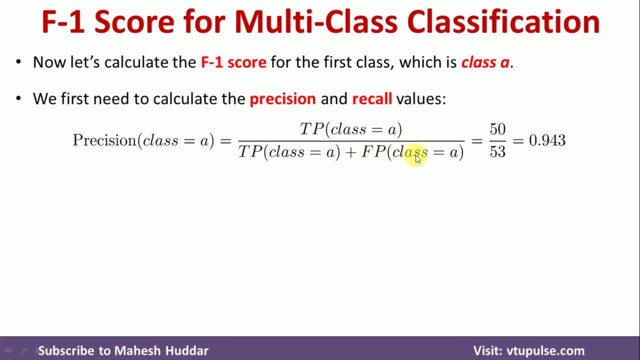 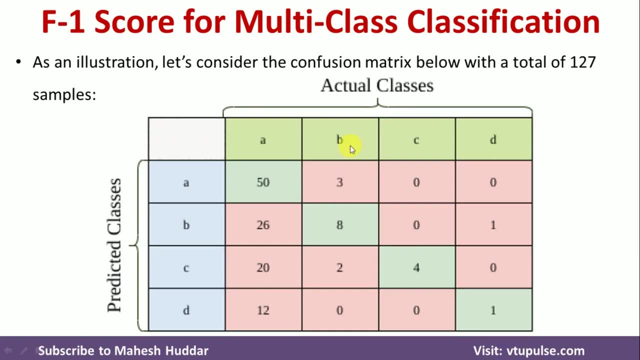 this one. one more number That is false positive when class is equivalent to A. False positive is this number, That is, 3, are of type B, but they were classified as A. The meaning is it's a false positive when class is equivalent to A. Again, 0 and. 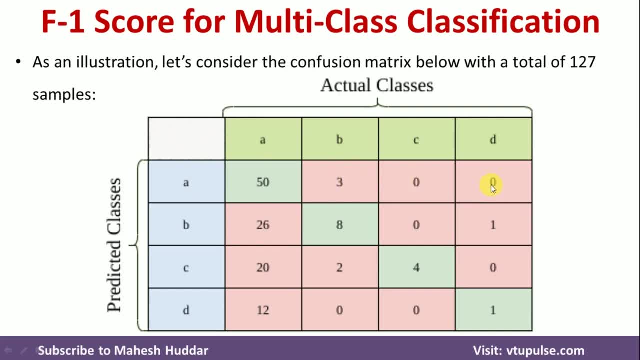 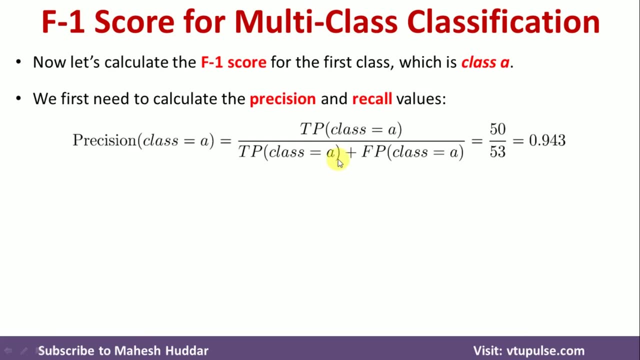 0 are also false positive. If I add all these things, it will become a false positive in this case. So, numerator, we will get 50 divided by true positive. again 50 plus 3 plus 0 plus 0. That is nothing but 50 divided by 3.. That is the precision when class is equivalent to A here. 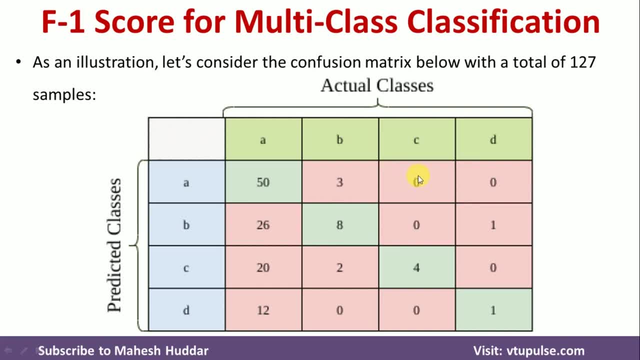 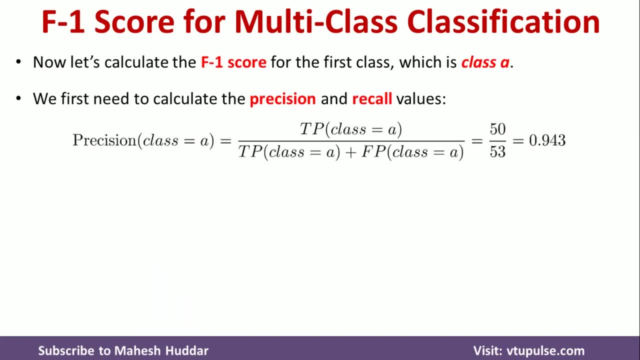 understand which is false positive and which is false negative here. now what we do is we will consider each class at a time and then we will try to calculate the f1 score here. now, if i consider the class a, first we need to calculate the precision recall for class a. that is the precision. 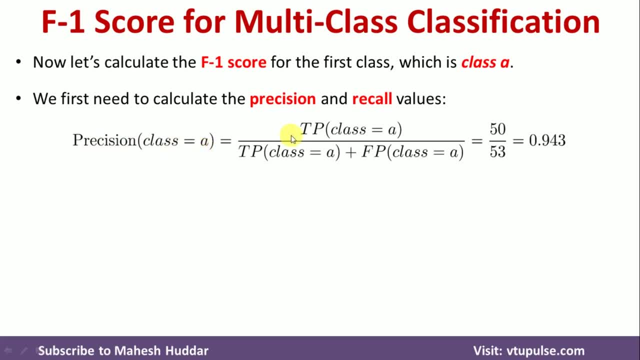 of class a is true positive when class is equivalent to a divided by true positive when class is equivalent to a, plus false positive when class is equivalent to a. so this is a formula to calculate precision: that is true positive divided by true positive plus false positive. but we have 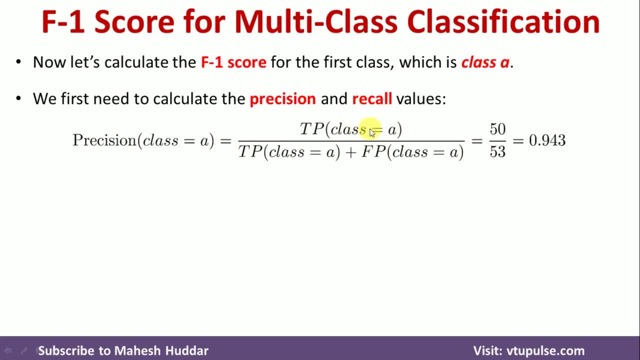 to specify when class is equivalent to a here. so this is a formula to calculate precision. that is true positive divided by true positive plus, because we have to calculate the f1 score individually. now what is true positive when class is equivalent to a is: if you look at this particular thing, this one, this 50 is nothing but. 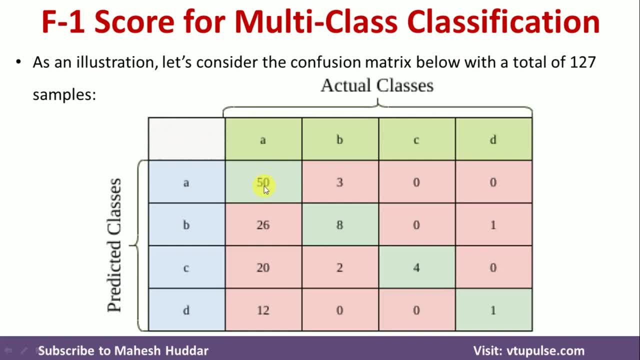 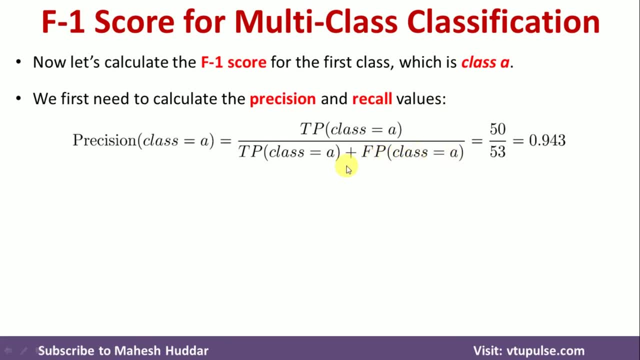 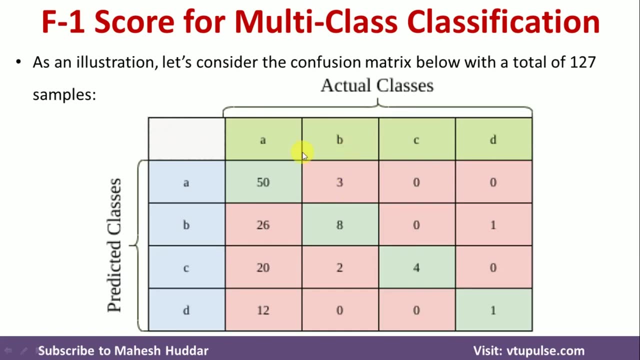 the true positive when class is equivalent to a, and what we need is this one: one more number that is a false positive when class is equivalent to a. false positive is this number, that is, three, are of type b, but they were classified as a. the meaning is: it's a false positive when class is. 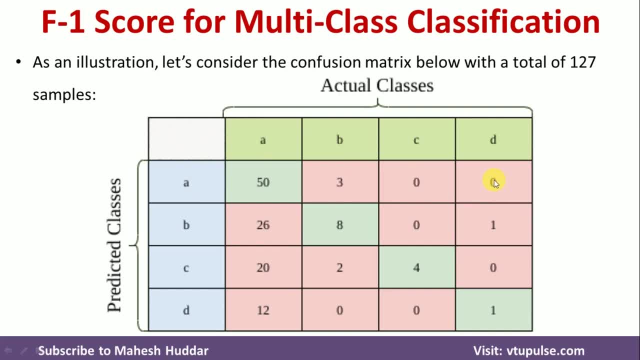 equivalent to a. again 0 and 0 are also false positive. if i add all these things, it will become a false positive in this case. so, numerator, we will get 50 divided by true positive. again 50 plus 3 plus 0 plus 0, that is nothing but 50 divided by 3. that is the precision when class. 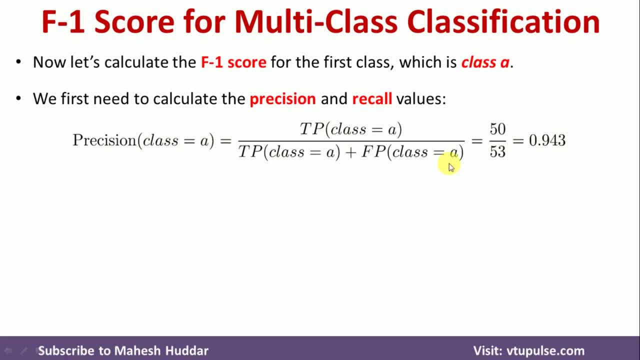 is equivalent to a here, so that is equal to 0.943 here. similarly, when it comes to the other one, that is recall, when class is equivalent to a, the formula is true positive divided by true positive plus false negative. now. so true positive: we already know that is 50. this true positive is again 50. what is false negative? 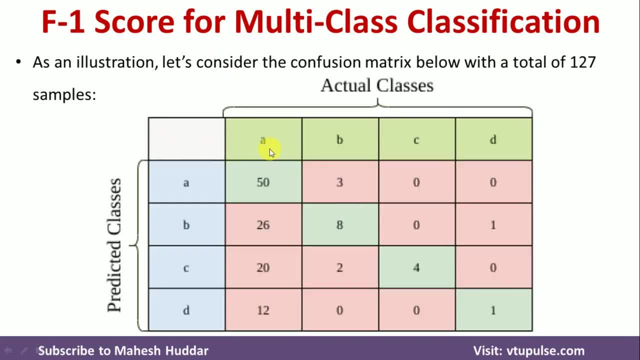 we have to check it out. false positive when class is is equivalent to a is that is 26, because the 26 examples are of type a, but they are false positive when class is equivalent to a. is this right? even in this case? let me see double. 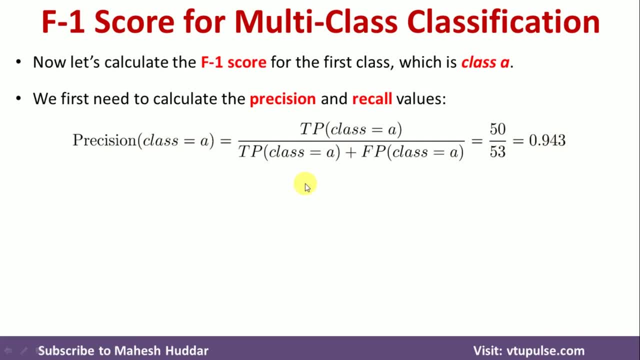 So that is equivalent to 0.943 here. Similarly, when it comes to the other one, that is recall, when class is equivalent to A, the formula is true positive divided by true positive plus false negative. now, So true positive, we already know that is 50.. This true positive is again 50.. What is false negative? 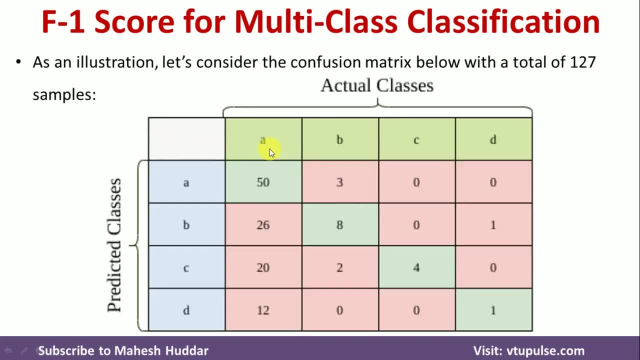 We have to check it out. False positive, when class is equivalent to A, is That is 26, because the 26 examples are of type A but they were classified as B. Similarly, 20 examples are of type A. They were classified as C. 12 examples are of type A, but they were classified as. 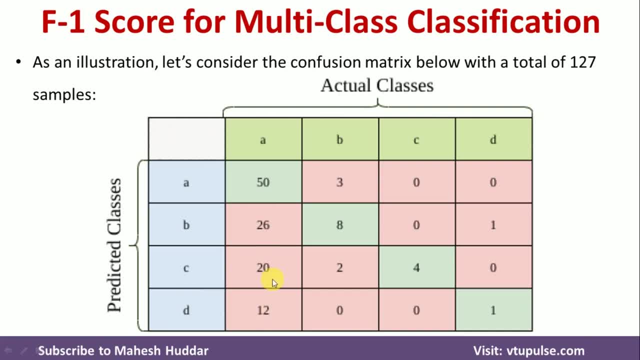 D here. So all these things are false, negative. in this case That is 26 plus 20 plus 12. in this case, That is nothing but 26 plus 20 is 46 plus 12 is 58 here. So the answer is: 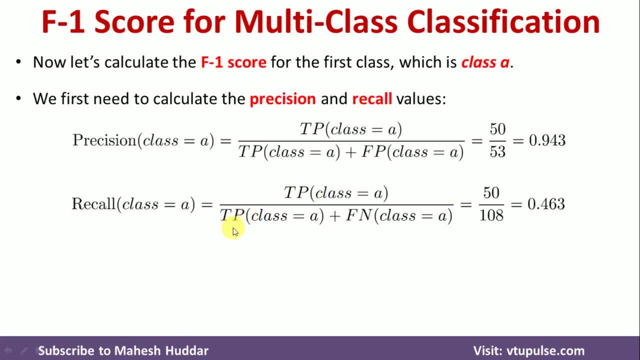 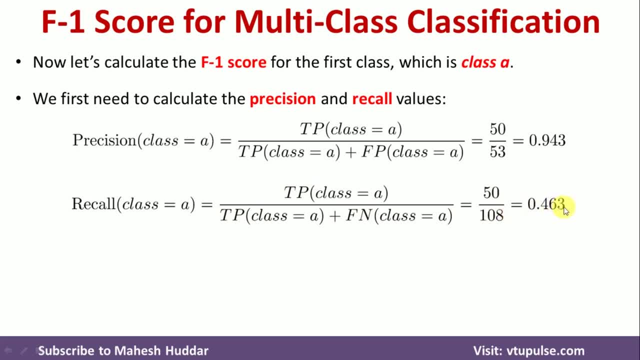 50 divided by 108, which is equivalent to 0.463 here. Now, once you calculate this precision recall, we can calculate the F1 score when class is equivalent to A. That is nothing but 2 times precision when class is equivalent to A multiplied by recall. when class is equivalent to A divided by, 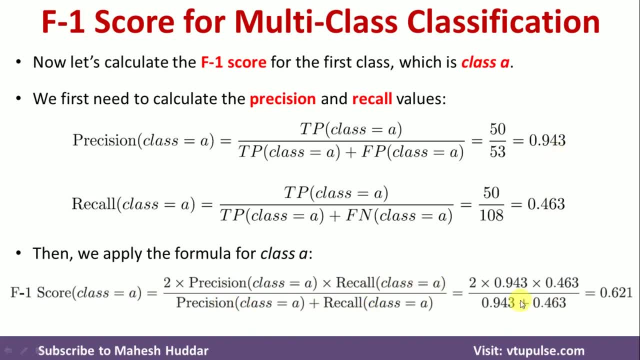 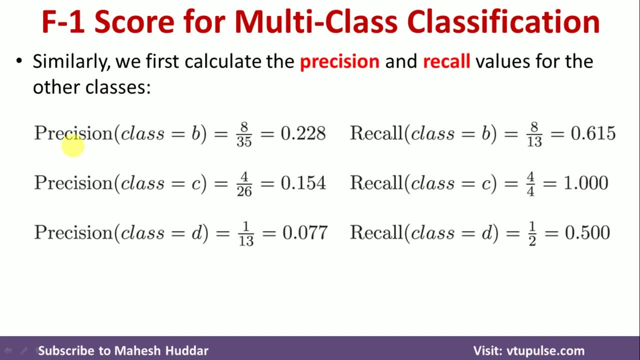 precision plus recall. So if you put this particular values in this equation, you will get the F1 score as 0.621 when class is equivalent to A. here, Similarly, we have to find the precision and recall for all the classes separately. Here I have shown: the precision when class is equivalent to B is 0.228, and recall when 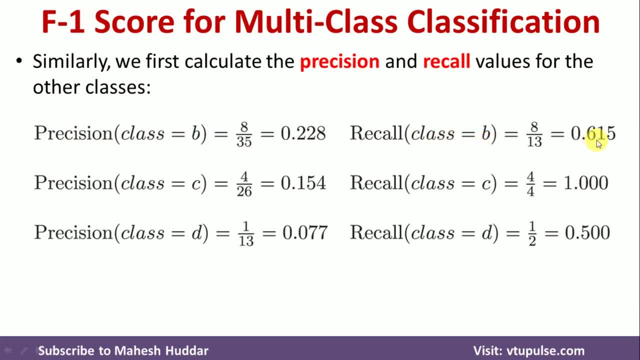 class B is equivalent to B is equivalent to 0.615.. Precision when class is equivalent to C is 0.154.. Recall when class is equivalent to C is 1.5.. Precision when class is equivalent to D is 0.077.. Recall when class is equivalent to D is: 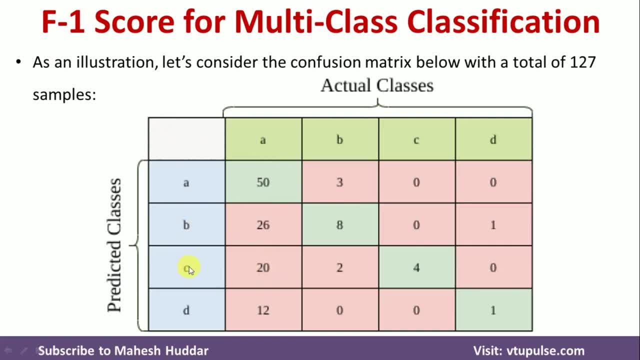 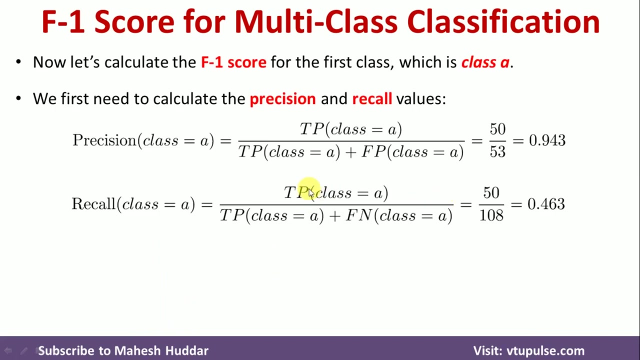 this is also similar: suits are false negative. So, Ano, this is today, but, but i will show a cops this day. i will show clear you: the more are true, positive and for this fn, we have 58. that is nothing but 50 divided by 108, which is equivalent. 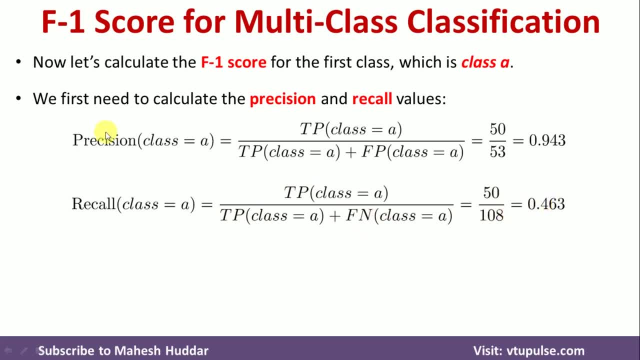 to 0.463 here. now, once you calculate this precision recall, we can calculate the f1 score. when class is equivalent to a, that is nothing but two times precision. when class is equivalent to a multiplied by recall, when class is equivalent to a divided by precision plus recall. so if you put 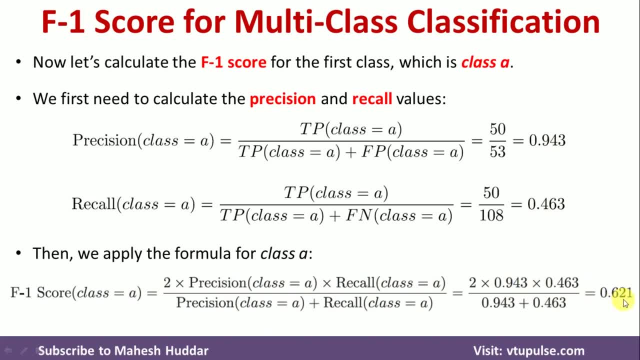 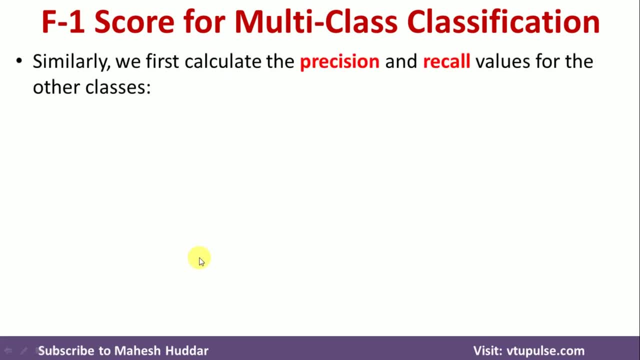 this particular values. in this equation you will get the f1 score as 0.621 when class is equivalent to a. here, similarly, we have to find the precision and recall for all the classes separately. here i have shown: the precision when class is equivalent to b is 0.228, and recall when class b is equivalent. 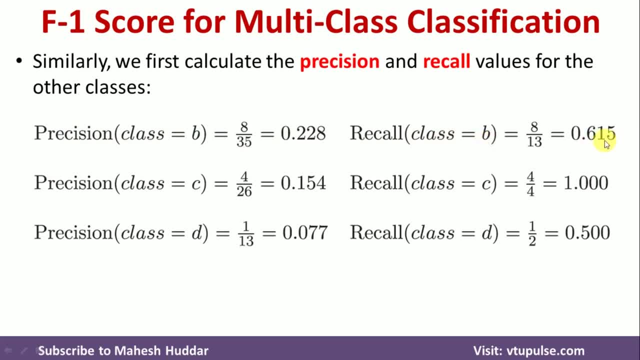 to b is equivalent to 0.615. precision when class is equivalent to c is 0.154. recall when class is equivalent to c is 1.0. precision when class is equivalent to d is 0.077. recall when class is equivalent to d is equivalent to 0.5. 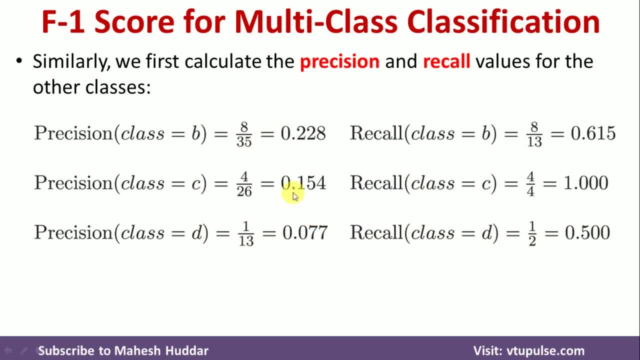 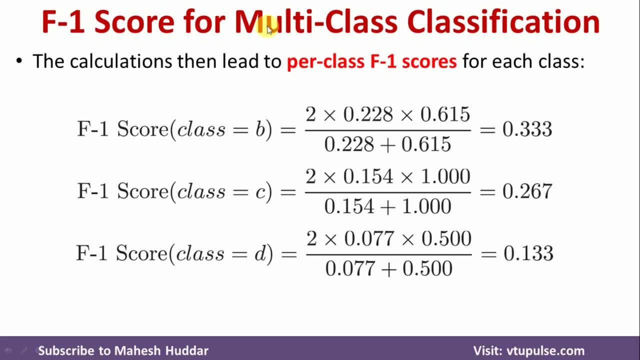 so once you know the precision and recall for every class, you can calculate the f1 score for individual classes, that is, we have already calculated. the p1 k when class is equivalent to b is By adding the pre fors plus thempref when class is equivalent to b, that gives us the hereon tíd: no. 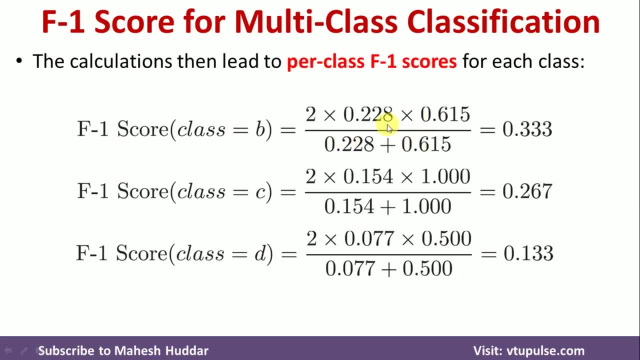 and youestä round is f1. we get the f1 score when class is equivalent to IBبi is two times precision multiplied by recall, divided by precision plus recall. when class is equivalent to B, b- we have already calculated these numbers. use these particular numbers in this equation. you will lack a wrong score. when class is equivalent to b, class is equal to see and class is equal to be. in this case, we got f1 score when class is equivalent to be as 0.거야2, etc. 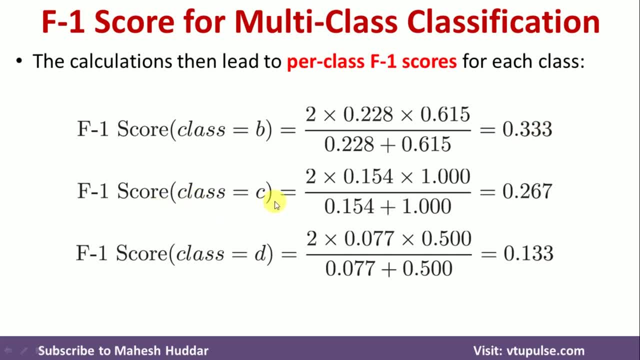 0.333.. F1 score when class is equivalent to C as 0.267.. F1 score when class is equivalent to D as 0.133 here. So this is a simple process we need to follow to calculate the F1 score. 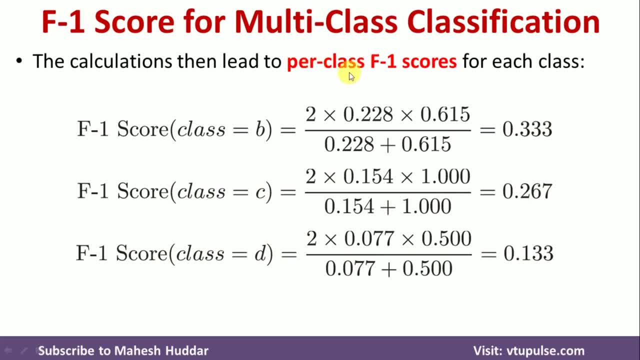 for multi-class classification. One point you can remember here: when it comes to binary classification, we will get overall F1 score, that is, one F1 score for the entire data set. but when it comes to F1 score for multi-class classification, for every class we have to. 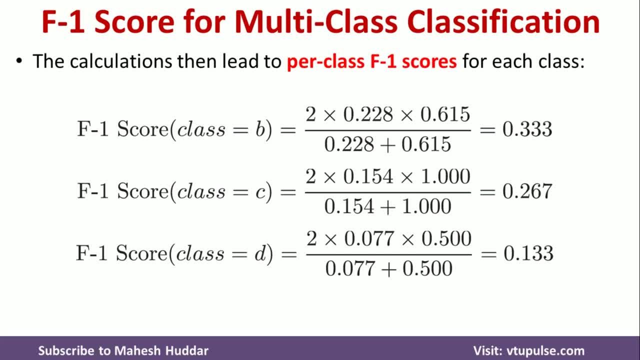 calculate the F1 score separately, by considering one versus rest in this case. So in this video we have understood how to calculate the F1 score for multi-class classification. If you like the video, do like and share with your friends. Press the subscribe button. 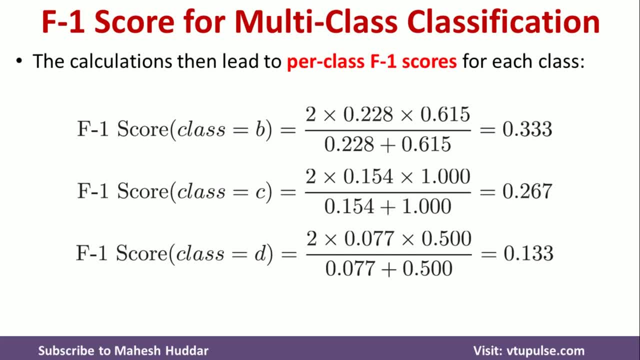 For more videos. press the bell icon for regular updates. Thank you for watching. 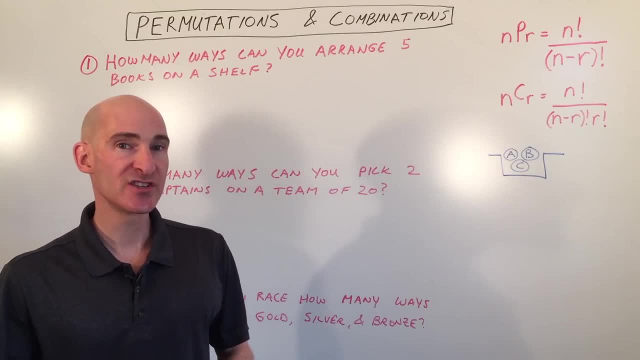 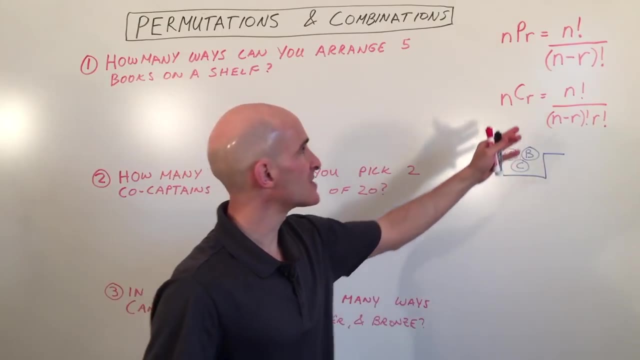 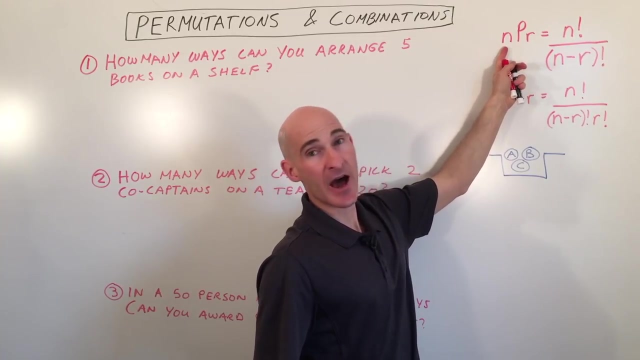 So what is a permutation? Well, basically what a permutation is? it's an ordering of a group of objects, And we'll take a look at some examples in a little bit. but first let's take a look at some formulas. here, What we have is NPR, which is basically out of N items. 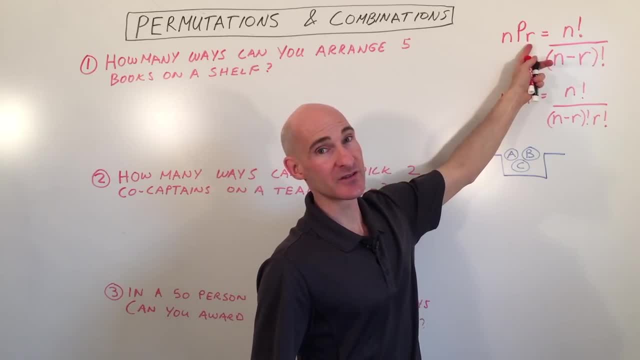 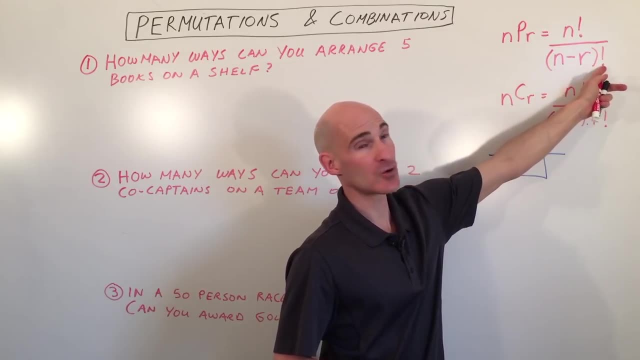 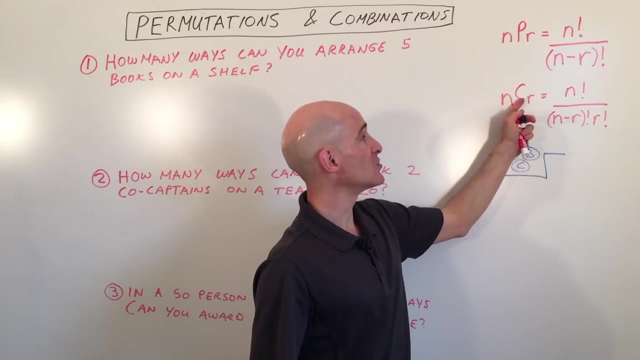 how many ways can you pick R items where the order is important? So the formula is N factorial over N minus R factorial, whereas combinations NCR out of N total items. how many ways can you choose R items where the order is not important? And I'll show you an example in. 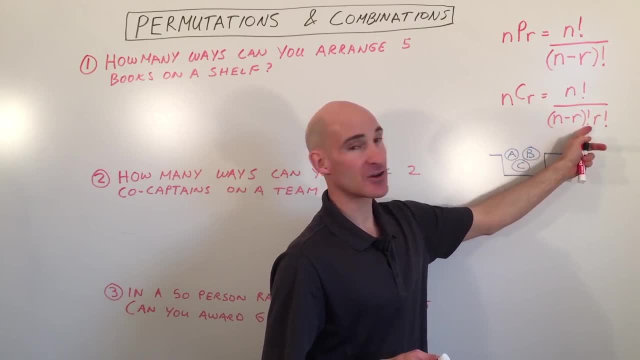 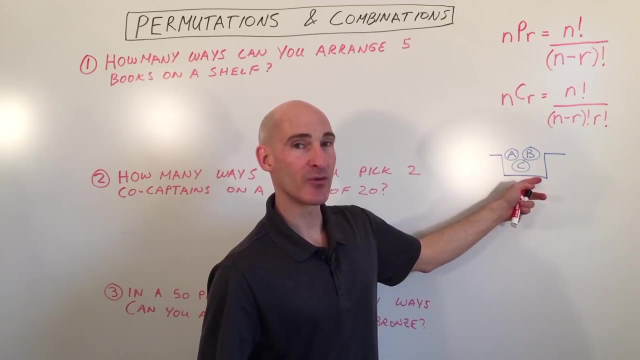 just a minute. but this formula is N- factorial over N minus R factorial- R factorial. Okay. so take a simple example like: say, you have a hat with three marbles in it- A, B and C- And you just want to pick a hat with three marbles in it- A, B and C- And you just want.